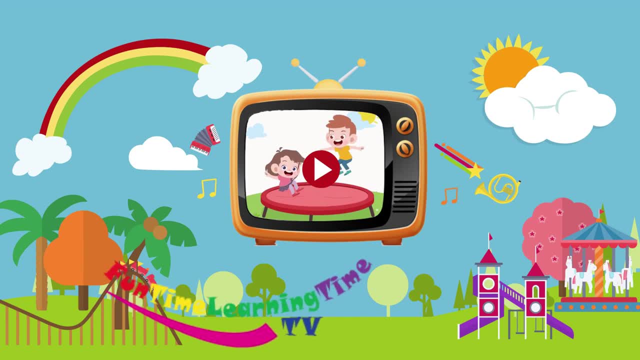 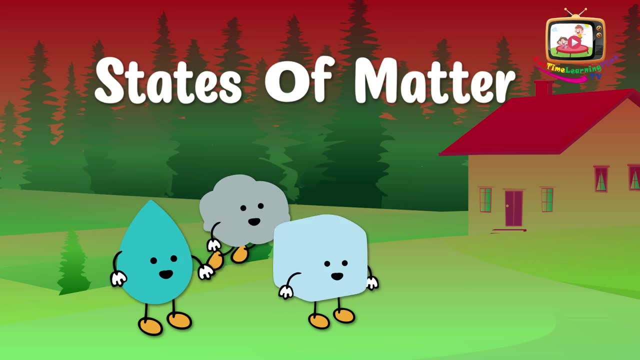 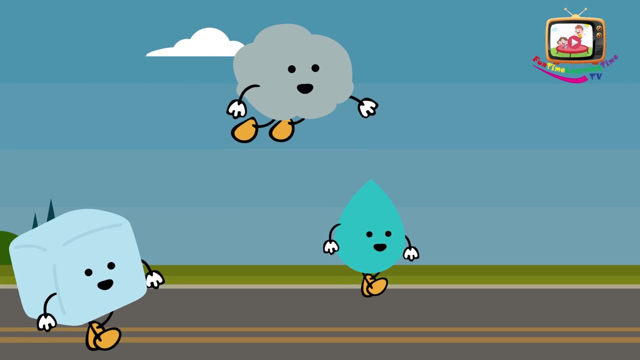 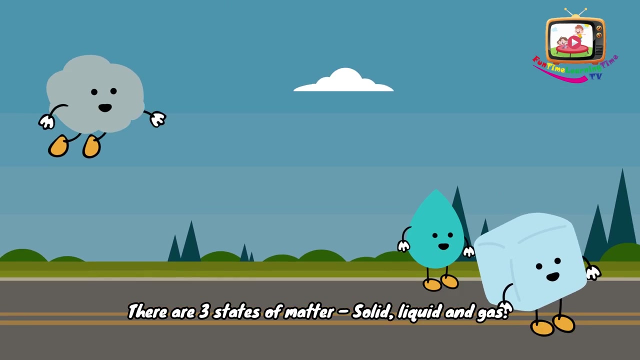 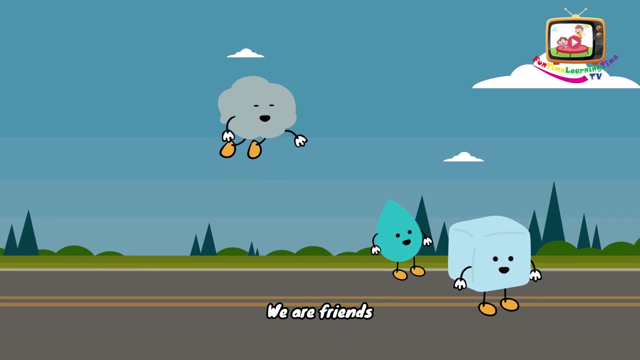 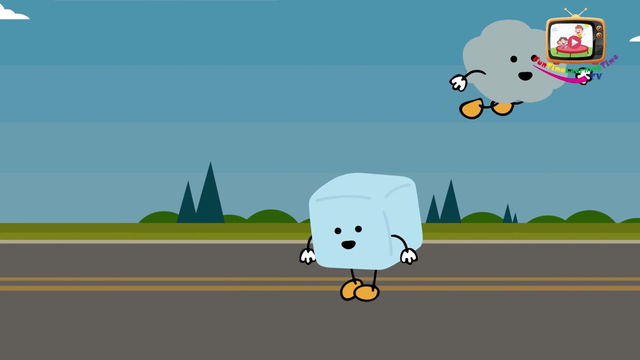 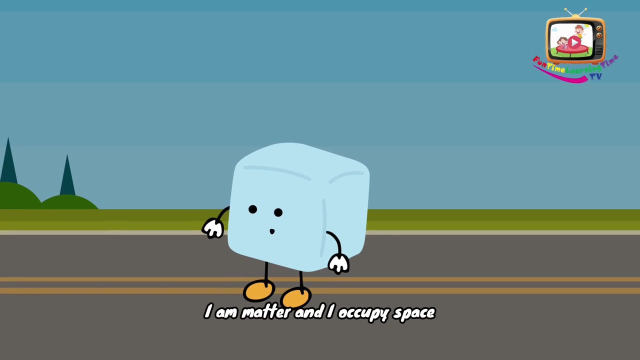 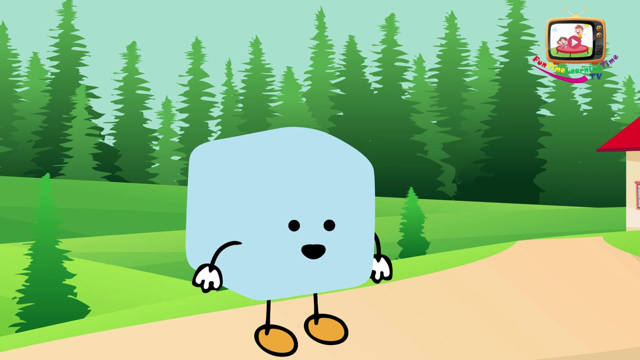 There are three states of matter: Solid, liquid and gas. We are friends. We can change state from one to another. I am solid, I am matter and I occupy space. My particles are tightly packed. You can touch me and I can be soft or hard. I have a shape and I can change state. 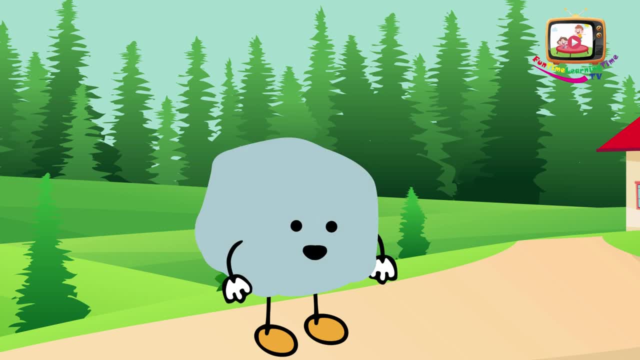 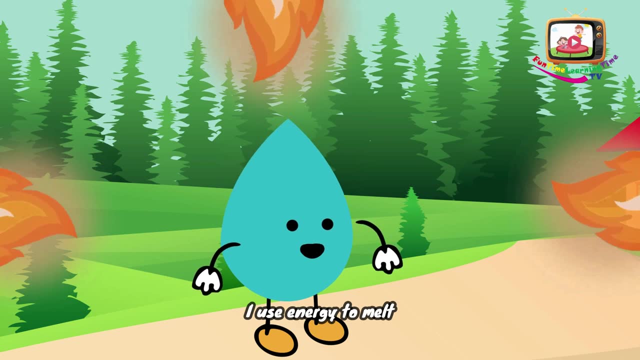 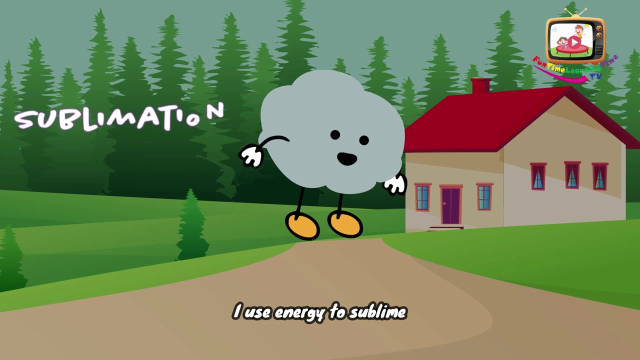 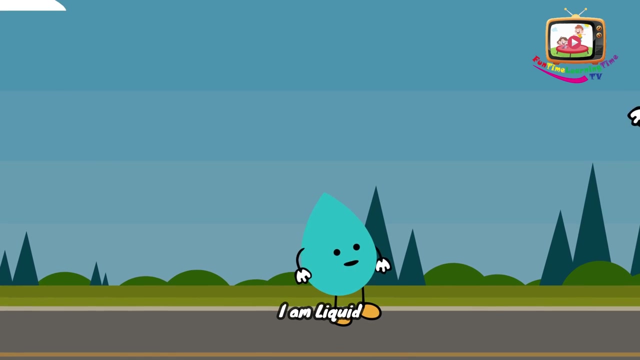 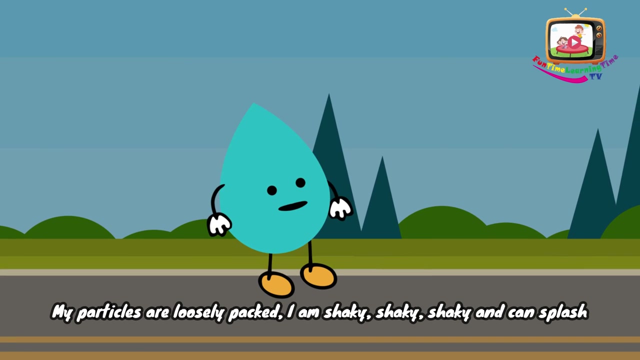 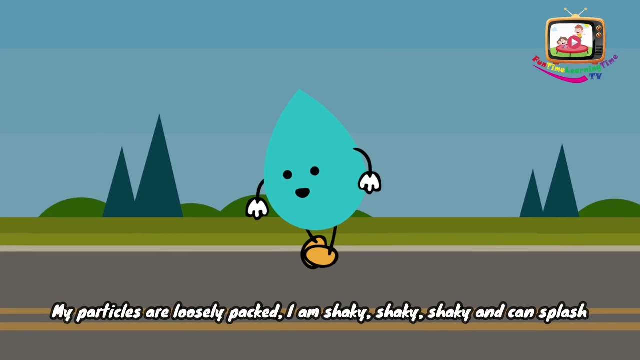 To liquid or gas. Melting changes me from solid to liquid. I use energy to melt. Sublimation change me from solid to gas. I use energy to sublime. I am liquid, I am matter and I occupy space. My particles are loosely packed. I am shaky, shaky, shaky and can splash. 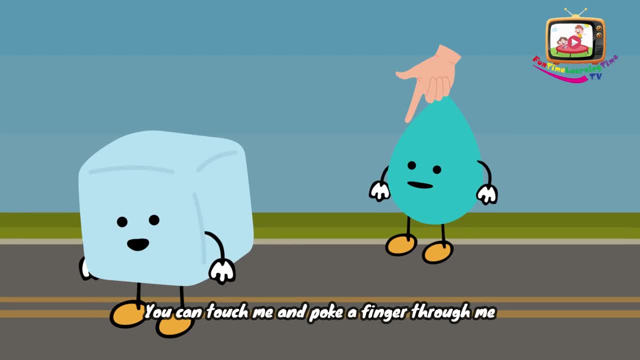 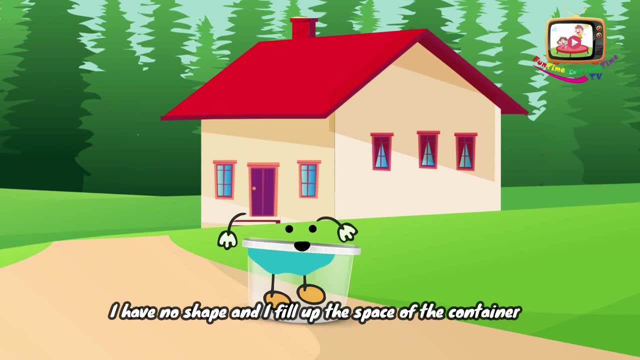 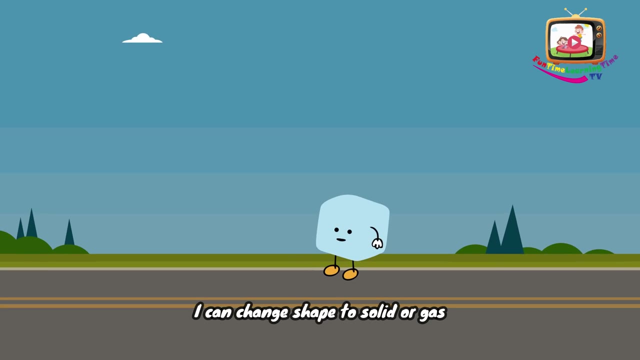 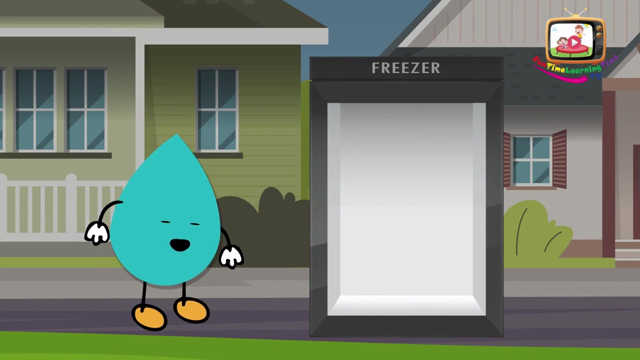 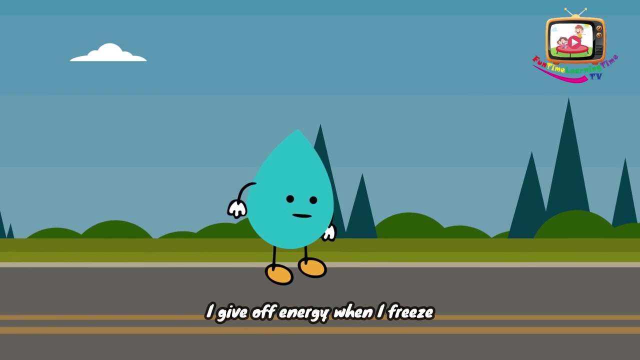 You can touch me and poke a finger through me. I have no shape and I fill up the space Of the container. I am matter and I occupy space. I can change shape to solid or gas. Freezing changes me from liquid to solid. I give off energy when I freeze. 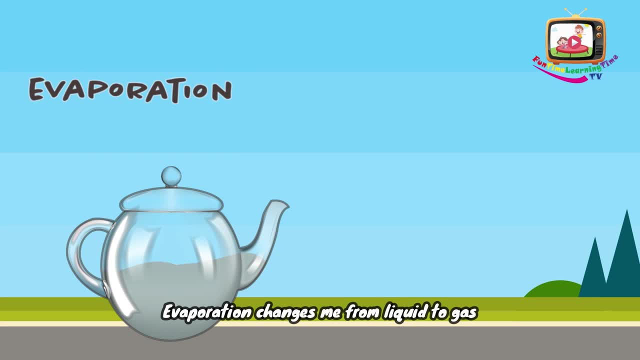 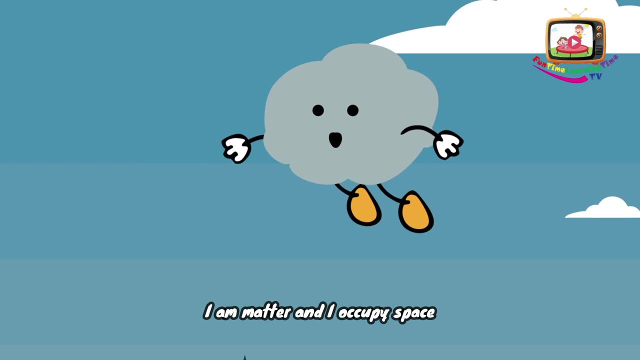 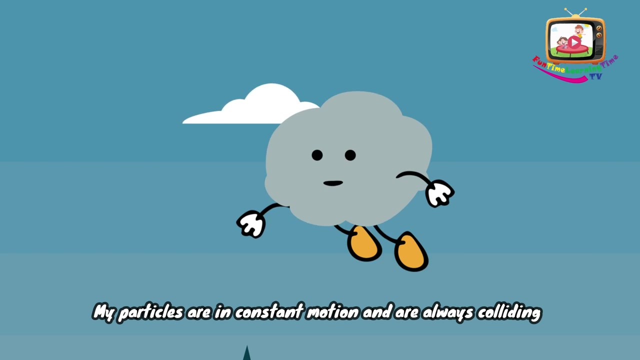 Evaporation changes me from liquid to gas. I use energy. when I evaporate, I am misguessing, I am matter and I occupy space. My particles are in constant motion And are always colliding. You can touch me, but I am compressible. I have no shape and I fill up the container.